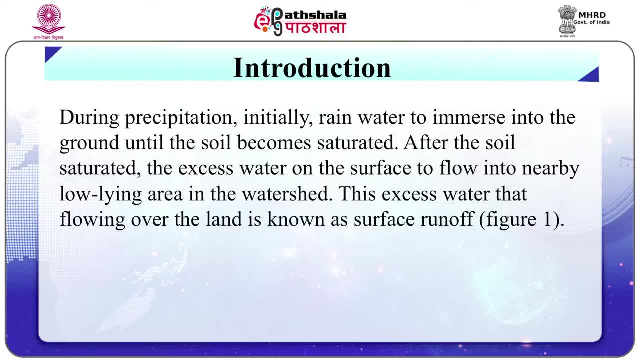 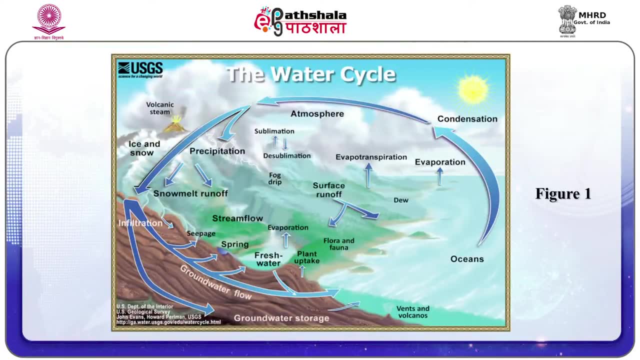 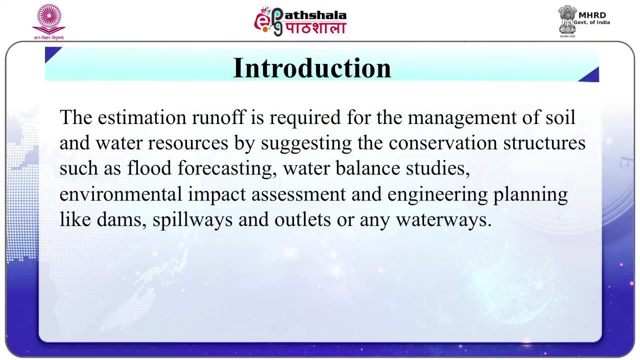 saturated. After the soil is saturated, the excess water on the surface to flow into nearby low lying area in the watershed. This excess water that flowing over the land is known as surface runoff, See the figure number 1.. The estimation of the runoff is required for the management of the soil and water resource by suggesting: 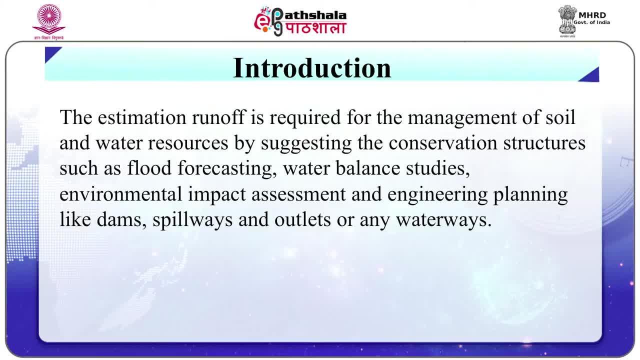 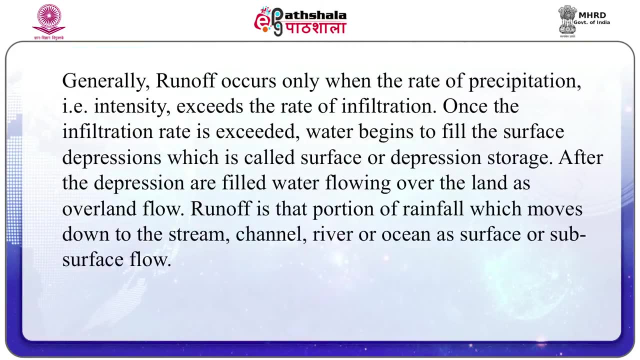 the conservation structure, such as flood forecasting, water balance studies, environmental impact assessment and engineering planning, like dams, spillway and outlet or any waterway. Generally, runoff occurs only when the rate of precipitation, ie intensity, exceeds the rate of infiltration. 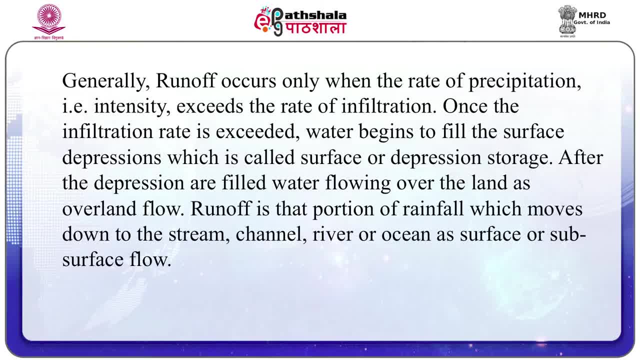 Once the infiltration rate is exceeded, water begins to fill the surface depression, which called surface or depression storage. After the depressions are filled, water flowing over the land as overland flow- Runoff- is the portion of rainfall which moves down to the stream, channel, river or ocean as surface or subsurface flow. Overland flow is the water. 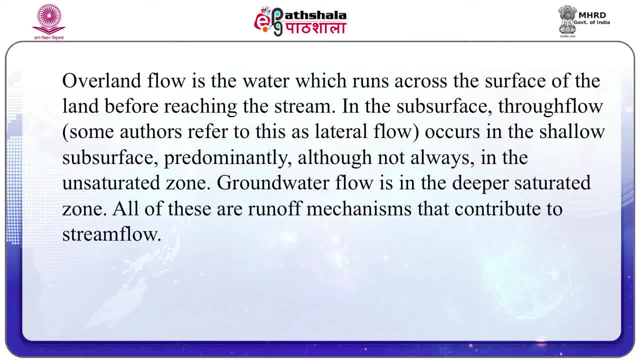 which runs across the surface of the land before reaching the stream In the subsurface through flow- some authors refer to this as lateral. flow- occurs in the shallow subsurface predominantly, although not always, in the unsaturated zone. Groundwater flow is in the deeper saturated zone. All these are runoff mechanisms that contribute. 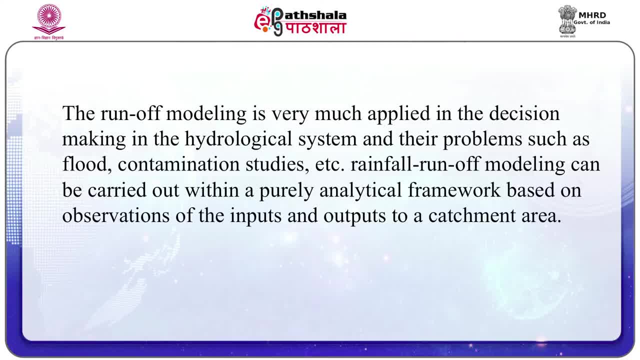 to stream flow. The runoff modeling is very much applied to the decision making in the hydrological system and their problems, such as flood contamination study, etc. Rainfall runoff modeling can be carried out within a pure analytical framework based on observation, input and output to a catchment area. The catchment is treated as a black box, without any reference to the water. 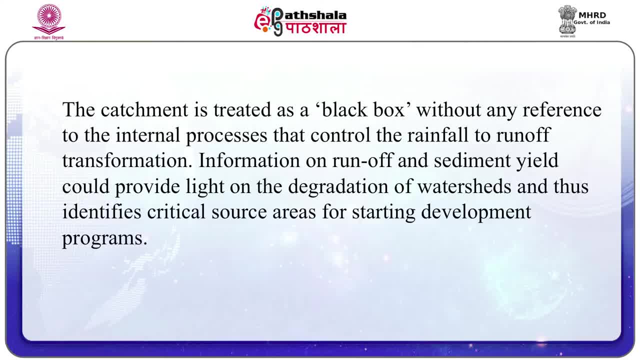 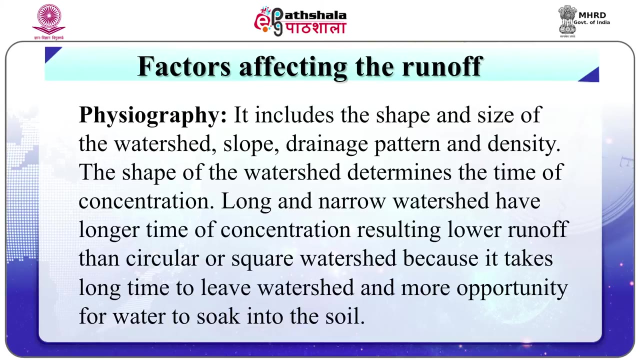 To the internal processes that control the rainfall to runoff transformation. information on runoff and sediment yield could provide light on the degradation of watershed and thus identify critical source area for starting development program. the factor affecting the rainfall Number 1 is Physiography. It includes the shape and size of the watershed. 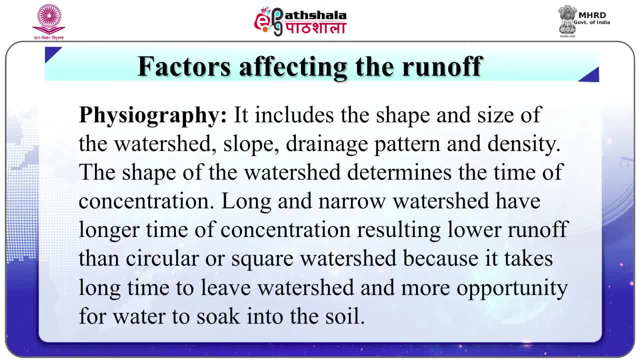 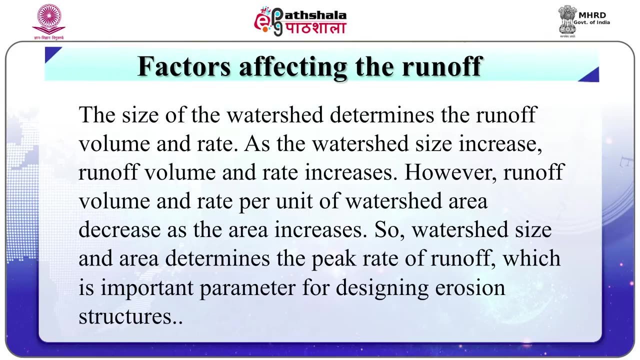 slope, drainage pattern and density. The shape of the watershed determine at the time of concentration. Long and narrow watershed have long time of concentration, resulting lower runoff than circular or square watershed, because it take long time to leave watershed and more opportunity to water to soak into the soil. The size of the watershed determine. 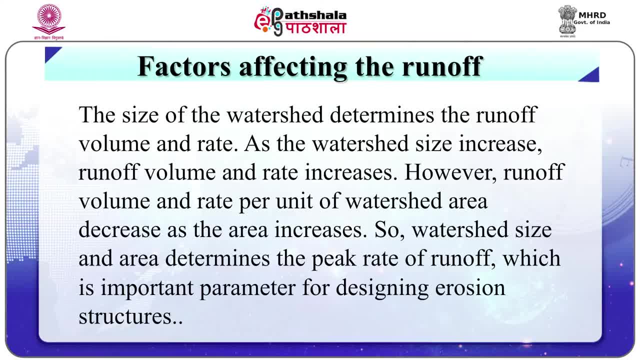 the runoff volume and rate as the watershed size increases. However, runoff volume and rate per unit of watershed area decreases as the area increases. So watershed size and area determines the peak rate of runoff, which is the important parameter for designing erosion structures. The slope of the watershed determines the 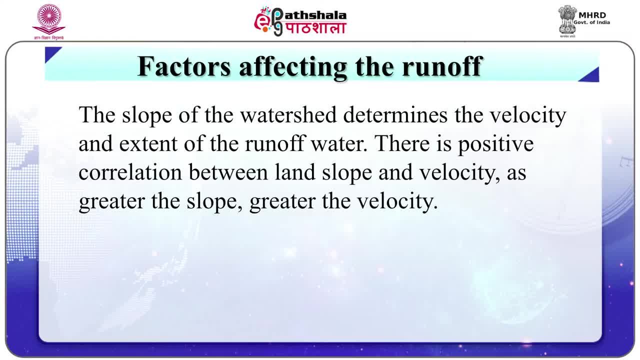 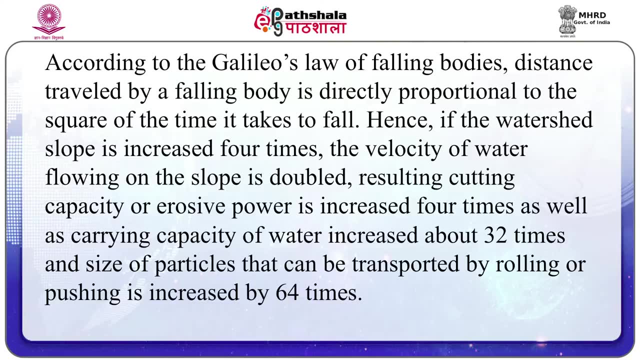 velocity and extent of the runoff water. Number 2 is Posture Positive correlation between land slope and velocity. As greater the slope, greater the velocity. According to the Galileo's law of falling body, distance travelled by a falling body is directly proportional to the square of the time it takes to fall. Hence, if the 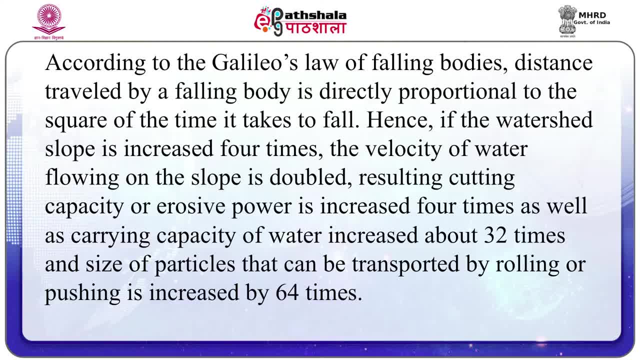 watershed slope is increased 4 times, the velocity of the water flowing on the slope is doubled, Resulting Carrying capacity, or erosive power, is increased 4 times, as well as carrying capacity of the water increased about 32 times and size of particle that can be transported by rolling. 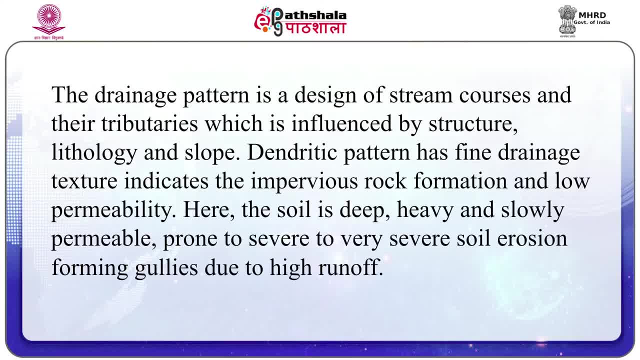 or pushing is increased by 64 times. The drainage pattern is a design of stream course and their tributary, which is influenced by structure, lithology and slope. Dendritic pattern has fine drainage texture. The drainage pattern is a design of stream course and their tributary, which is influenced by structure, lithology and slope. 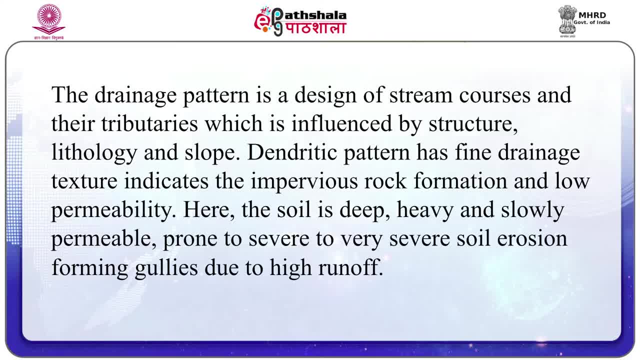 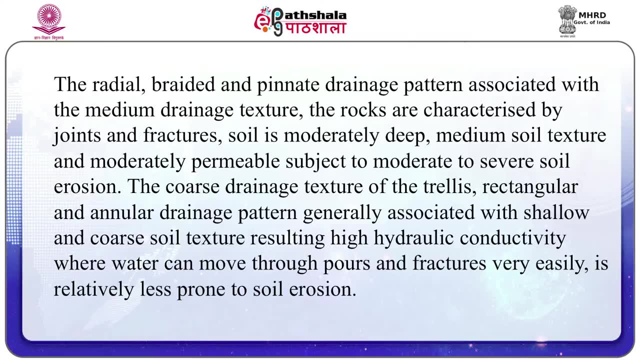 The drainage pattern of the soil is used to sand, making the soil smelly, faint, green or gheated. and here we better understand this Tambattering of the soil, scoop up vidare projections and the soil pH and greatly increase the yield horsepower. 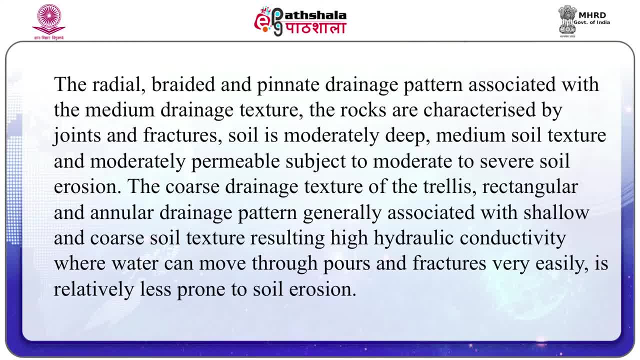 The drainage pattern is a design of skew blade as the base elected Rb. here are indicated The impervious rocks formation and low permeability. moderately deep medium soil texture and moderately permeable subject to moderate to severe soil erosion. The coarse drainage texture of the trellis rectangular and annular drainage pattern generally. 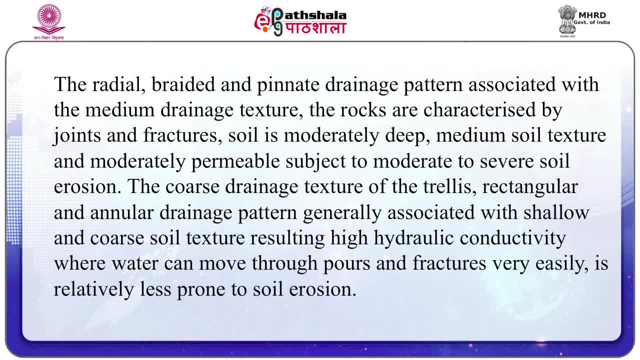 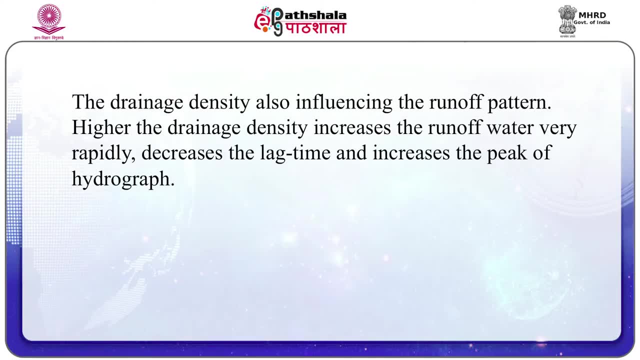 associated with shallow and coarse soil texture, resulting high hydraulic conductivity. where water can move through pore and fracture very easily, It relatively less prone to the soil erosion. The drainage density also influence the runoff pattern. Higher the drainage density, increase the runoff water very rapidly, decrease the lag time. 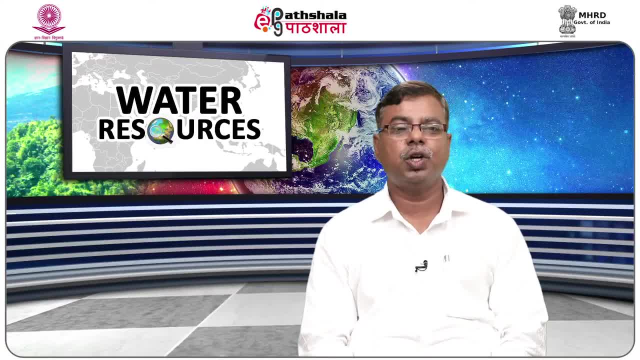 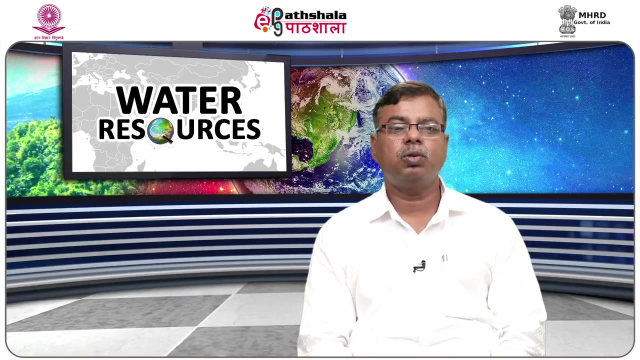 and increase the peak of hydrograph, Soil and Geology. The soil and geological characteristics determine the amount of saltation in the water, Water harvesting structure such as dam and reservoir, as well as amount of water percolated in the soil Precipitation. 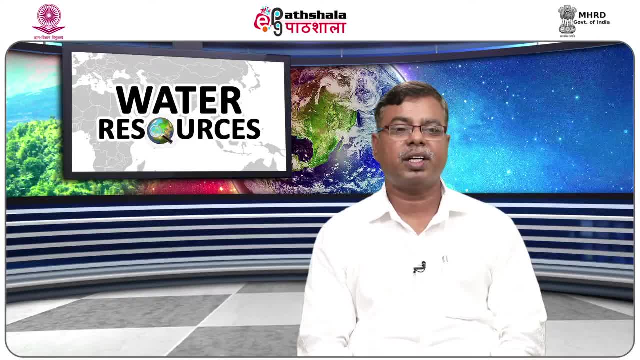 The amount and nature of precipitation is the most important factor which determine the runoff in a watershed: The quantity and rate of runoff. The quantity and the rate of runoff is prerequisite for the planning and designing of canal ditches or any other water harvesting structure. 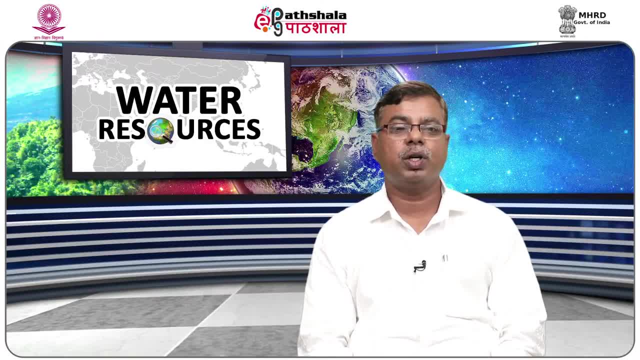 The volumetric assessment of water is most important. while impounding or creating reservoir, The rate of runoff is essential for conveying water from one place to another place by creating mechanical fracture to accommodate the flow of water. Theoretically, watershed with impervious rocks and no loss of water. maximum rate of runoff. 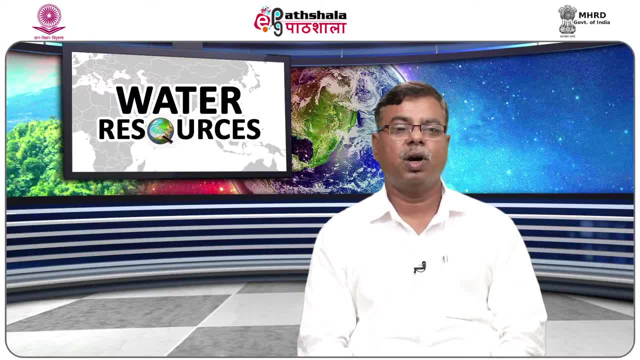 would be directly proportioned to the flow of water. Theoretically watershed with impervious rocks and no loss of water. maximum rate of runoff would be directly proportioned to the flow of water, Theoretically watershed with impervious rocks and no loss of water. so more the rainfall. 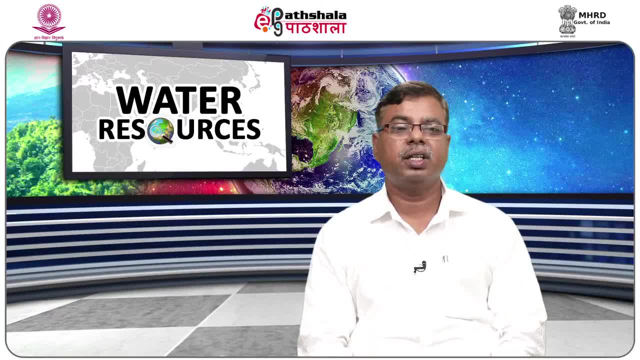 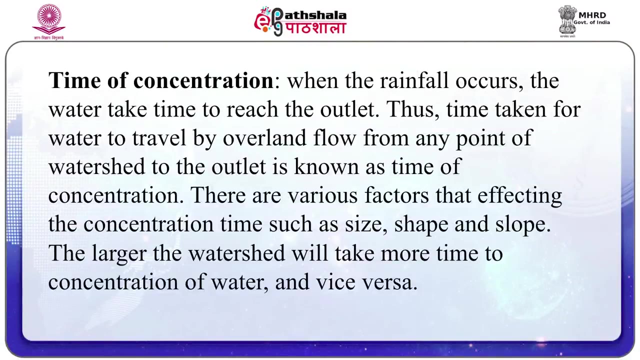 more runoff, But in the natural condition there are various interceptors, such as vegetation infiltration into the soil stored in depression, and some rainfall is evaporated. Therefore, estimation of rate of runoff depends on the rate of runoff and water available for runoff, Secret conditions and the time of consideration of rainfall. 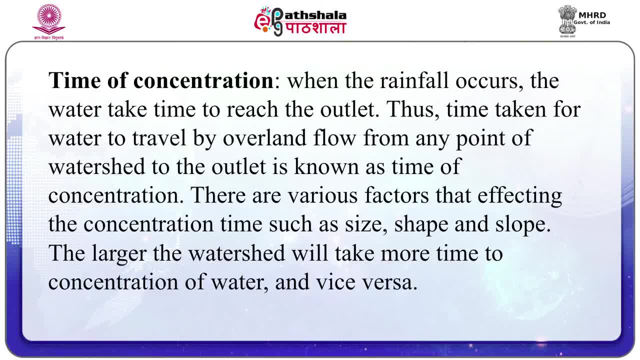 Soundman, The rainfall occurs, the water take time to reach the outlet. thus, time taken for water is travelled by overland flow from one point of watershed to the outlet is known as time of concentration. There are various factor that affecting the concentration time, such as size, shape and 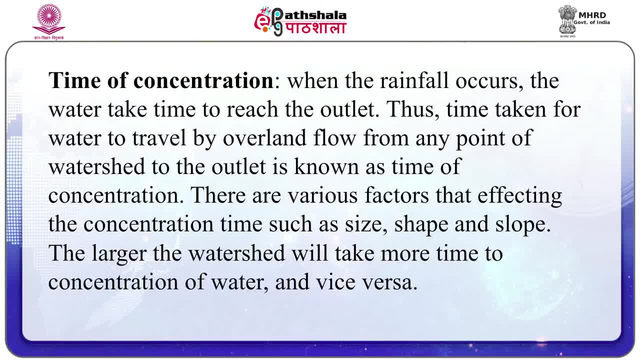 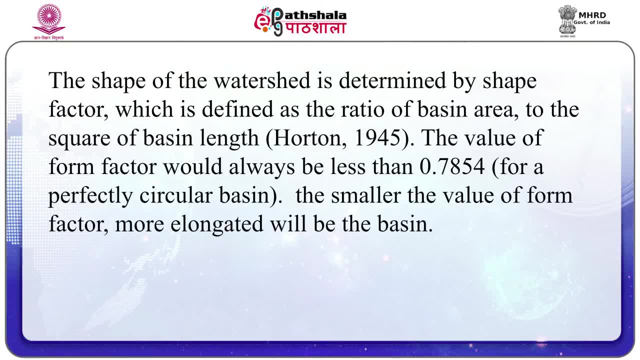 slope. The larger the watershed will take more time to concentration of the water, and vice versa. The shape of the watershed is determined by the Shea factor, which is defined as a ratio of basin area to the square of basin length. The value of form factor would always be less than 0.7854.. 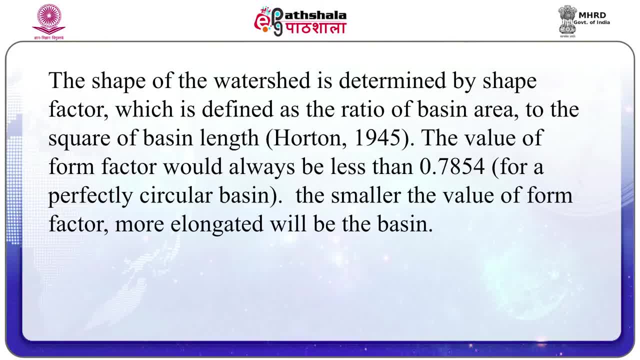 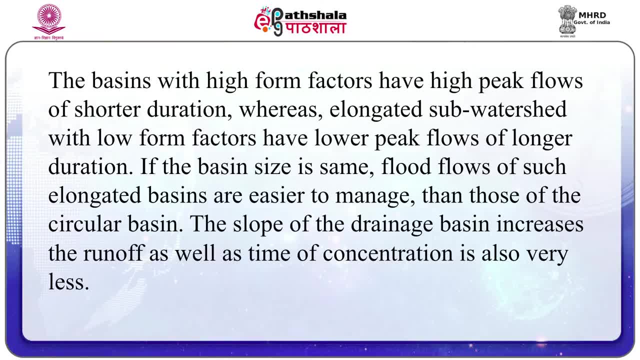 The smaller the value of form factor, more elongated will be the basin. The basin with high form factor have high peak flow of the shorter duration, whereas elongated sub-watershed With low form factor have low peak flow of low duration. If the basin size is same, flood flow in such elongated basin are easier to manage than 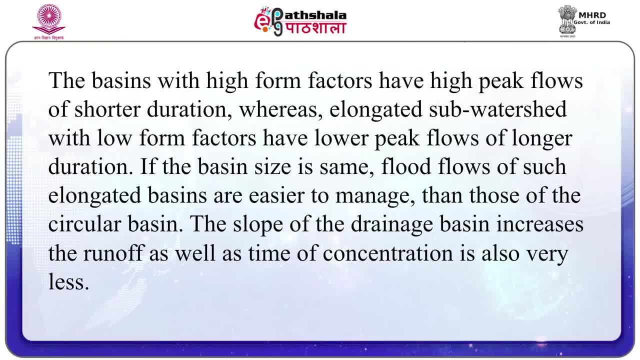 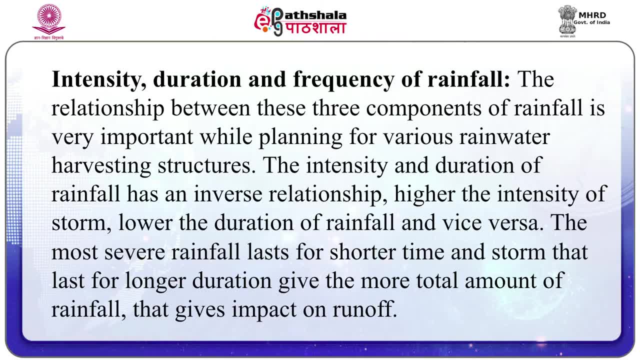 those of the circular basin. The slope of the drainage basin increases the slope as the time of concentration is very less. Intensity, duration and frequency of rainfall: The relationship between these three components of rainfall is very important while planning for various rain harvesting structure. 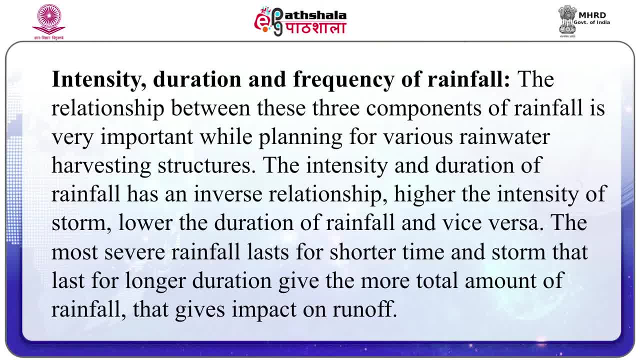 The intensity and duration of the rainfall has inverse relationship. Higher the intensity of the storm, lower the duration of rainfall and vice versa. The more severe rainfall last for shorter time and the storm that last for longer duration give the more total amount of rainfall that give impact on runoff. 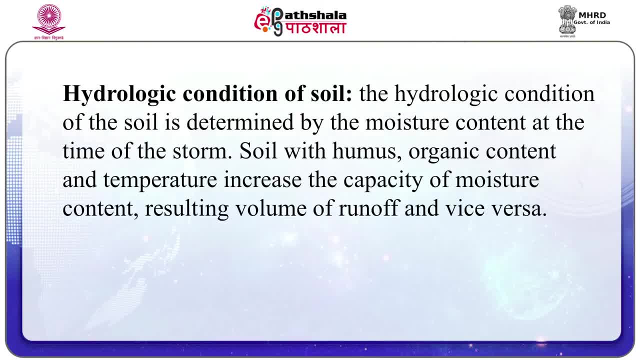 Hydrologic condition of the soil. The hydrologic condition of the soil is the determined by the moisture content at the time of the storm. Soil with humus, organic content and temperature increase the capacity of moisture content, resulting volume of runoff and vice versa. Vegetation cover. 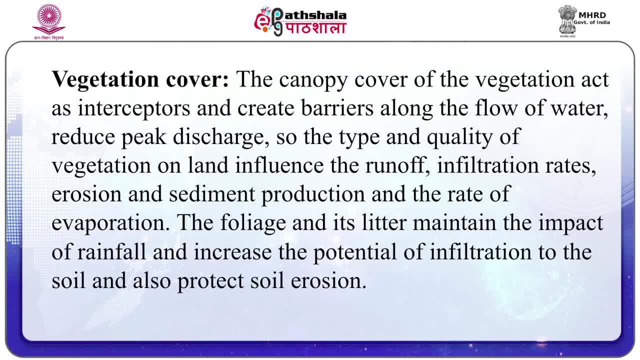 The canopy cover of the vegetation act as interceptor and create barrier along the flow of water, Reduce peak discharge. So the type of quality of vegetation on land influence the runoff infiltration rate, erosion and sediment production and the rate of evaporation. The foliage and it litter maintain the impact of rainfall and increase the potential of. 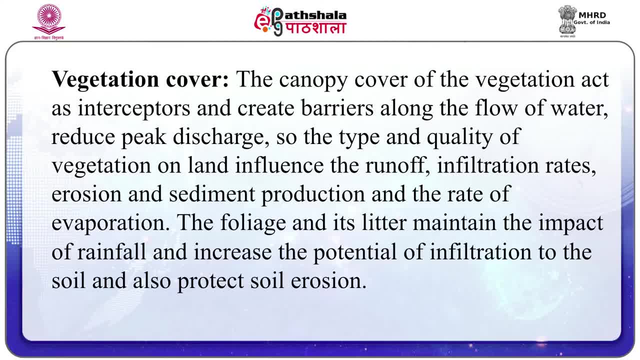 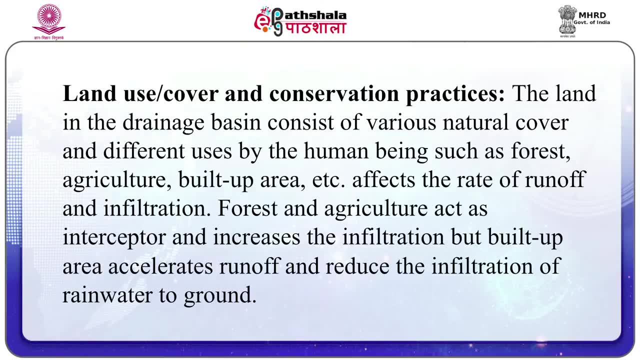 infiltration to the soil and the soil protect soil erosion. Thus the canopy cover and the ground litter create barrier to the water to flow on the land surface, Resulting increase time of concentration at it. reduce the peak discharge rate. The land use, land cover and conservation practices. 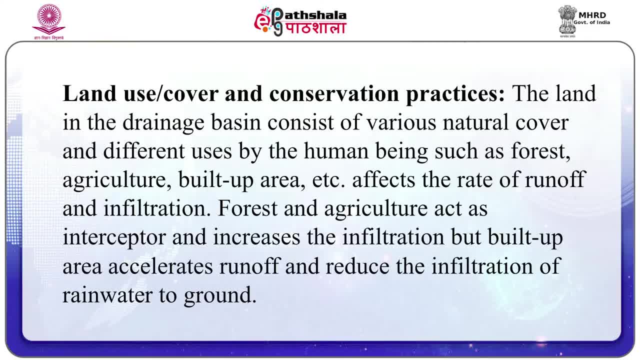 The land in the drainage basin consist of the various natural cover and different uses by the human beings, such as forest, agriculture, built up area, etc. Affecting the rate of runoff and infiltration. Forest and agriculture act as interceptor and increase the infiltration. 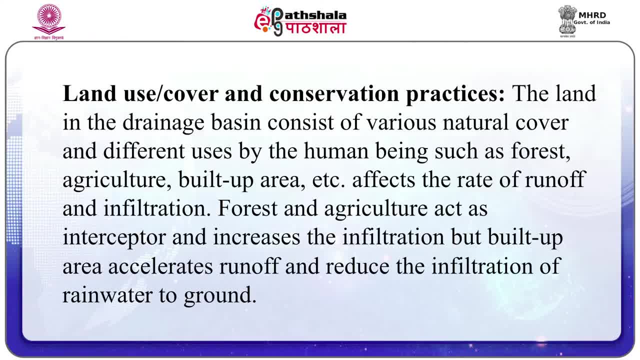 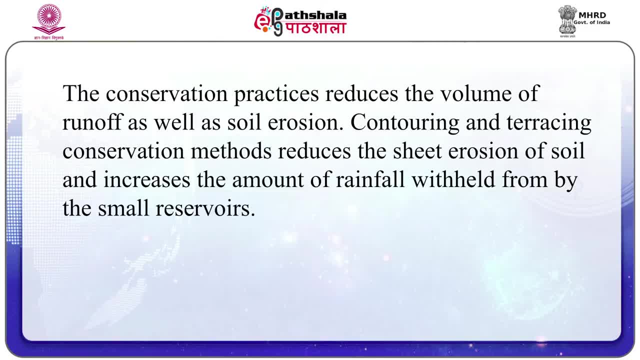 But Build up area, accelerate runoff and reduce the infiltration of rain water to ground. The conservation practice reduces the volume of runoff as well as the soil erosion. Contouring and terracing conservation method reduces the sheet erosion of the soil and increases the amount of rainfall withheld from the small reservoir. 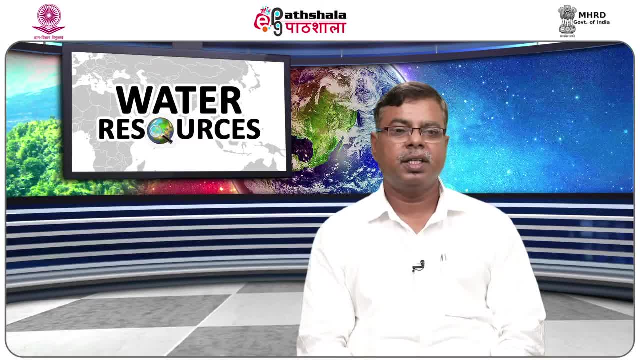 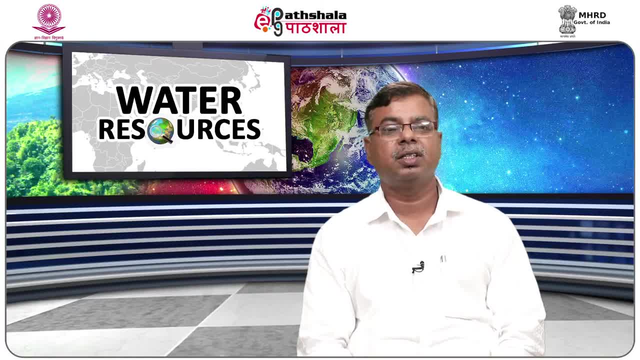 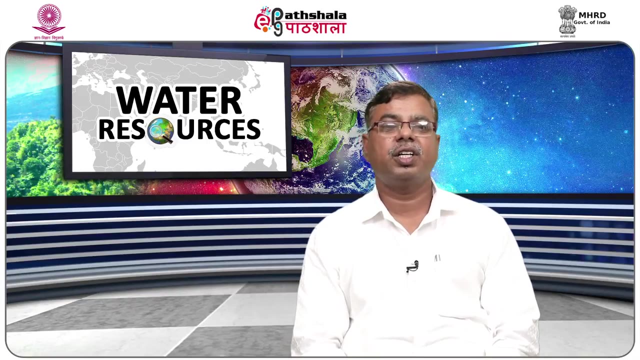 Which is suitable for small watershed, such as rational method, curve number method, cook method, table method and the hydrograph. For applying these method, two assumptions are made. One is rainfall occur with uniform intensity over the entire drainage basin and secondly, rainfall occurs at uniform intensity for duration at least equal to the time of concentration. 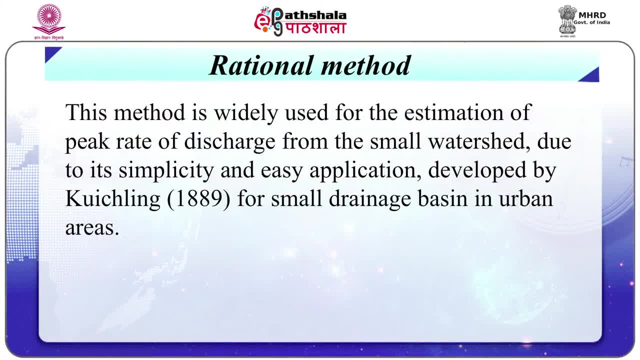 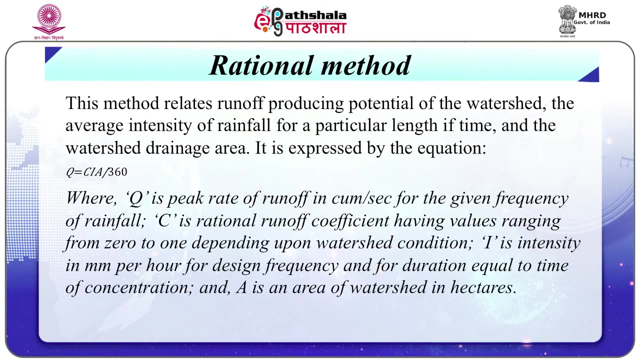 of the drainage basin. Number one: the rational method. This method is widely used for the estimation of peak rate of discharge from a small watershed due to its simplicity and easy application developed by Kuliching for small drainage basin in urban areas. This method relates runoff producing potential of the watershed. 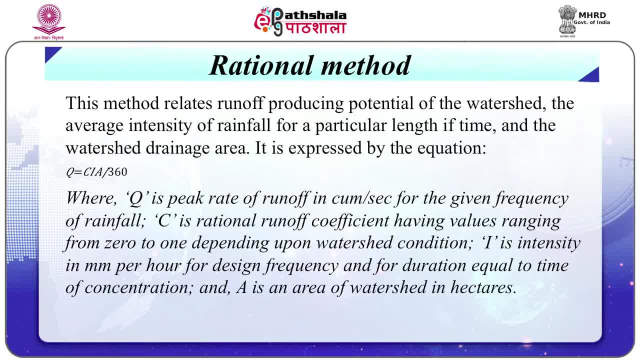 This method relates runoff producing potential of the watershed, The average intensity of rainfall for a particular length, if time, and the watershed drainage area. It is expressed by the equation: When catchment area with different value of c, the weighted value of c should be calculated. 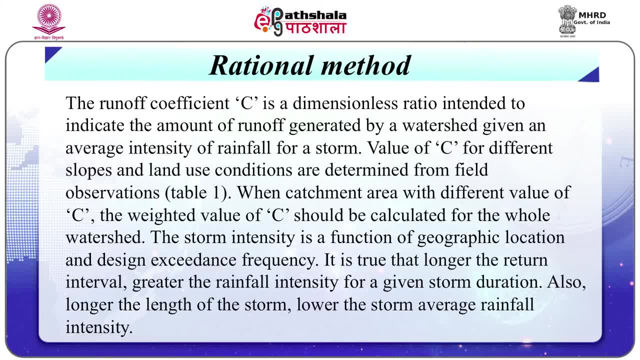 for the whole watershed. The storm intensity is a function of geographic location and design. Accidents frequency. It is true that longer the return interval, greater the rainfall intensity for a given storm duration. Also, longer the length of the storm, lower the storm average rainfall intensity. 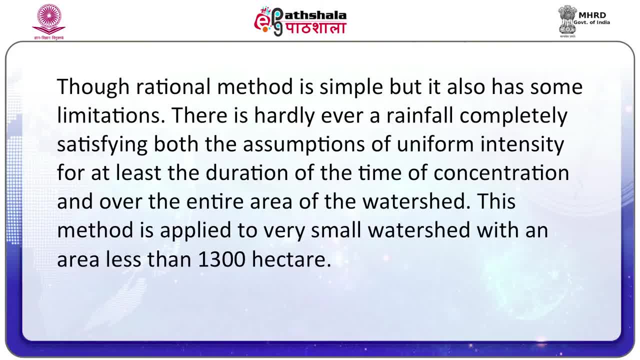 Though rational method is simple, but it is, but it also has some limitation. There is a hardly over a rain completely satisfy both the rainfall intensity and the rainfall intensity, The rain concentration of a time, Whether it is just the rain or is it peaks. 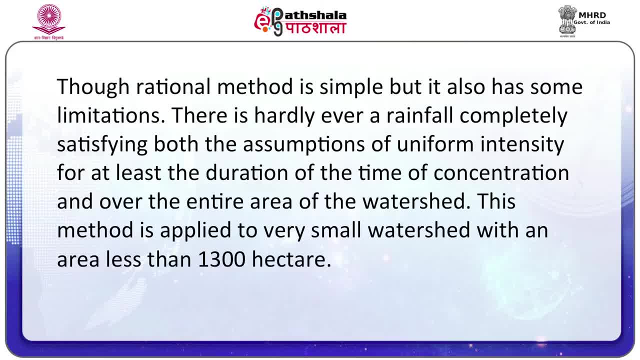 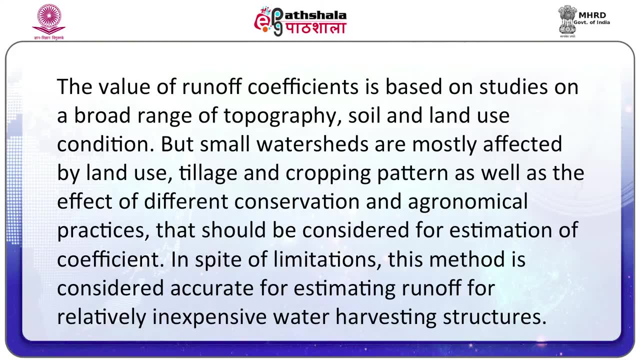 It is surely about the moving and the deviation. This method is applied to small watershed with an area less than 13000 hectares. The value of the runoff coefficient is based on the study on a broad range of topography, soil and land use conditions. 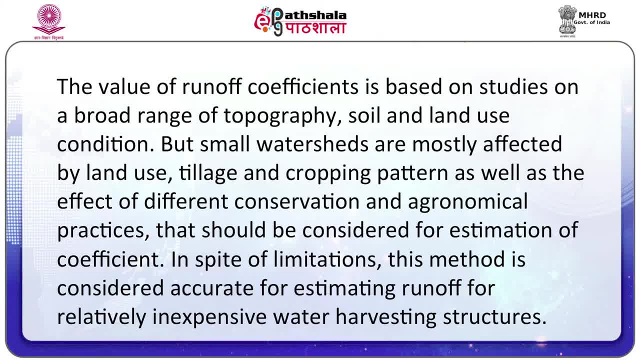 But a small watershed. It is one of the most effective models of more than three and third percent of the water. Kuliching for small management with less than 13000 hectares each year is a particular, affected by land use, tillage and cropping pattern, as well as the effect of different 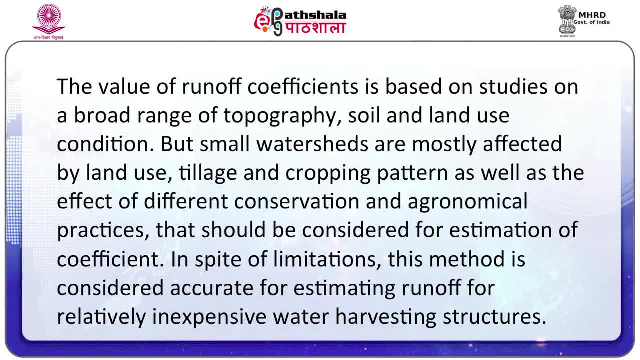 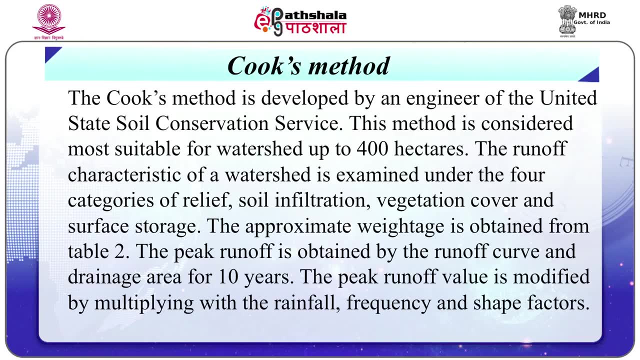 conservation and agronomical practices That should be considered for estimation of coefficient. In spite of limitation, this method is considered accurate for estimating runoff for relatively inexpensive water harvesting structures. Another method is Cook method. The Cook method is developed by an engineer of the United States Soil Conservation Services. 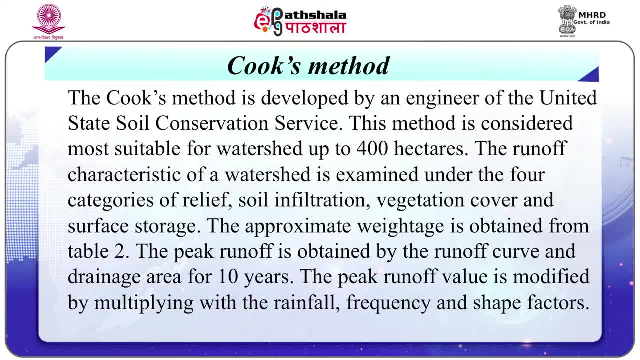 This method is considered most suitable for watershed up to 400 hectares. The runoff characteristics of a watershed is examined under the four categories of relief: soil infiltration, vegetation cover and surface storage. The approximate weightage is obtained from table 2.. The peak runoff is obtained by the runoff. 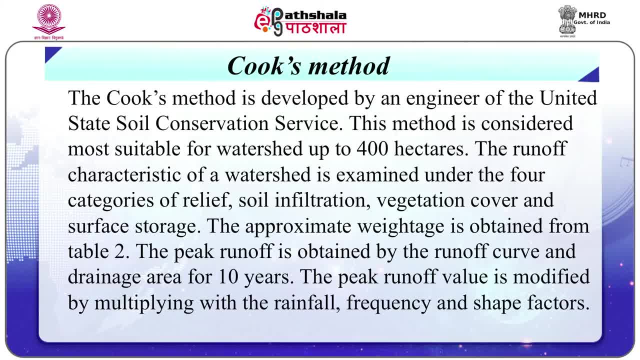 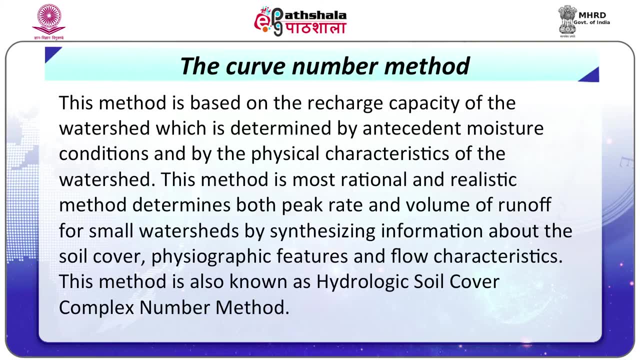 curve and the drainage area for 10 years. The peak runoff value is modified by multiplying the with rainfall frequency and shape factor. The another method is the curve number. This method is based on the recharge capacity of watershed, which is determined by the antecedent. 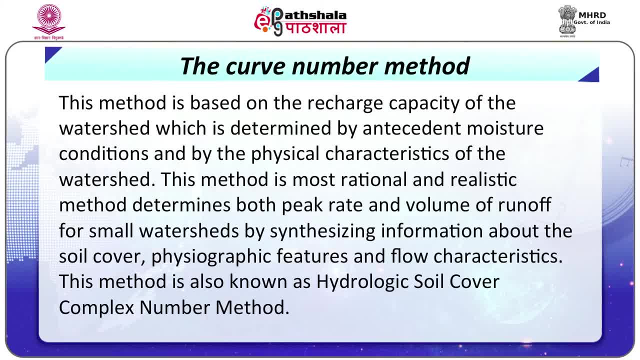 moisture conditions and by the physical characteristics of watershed. This method is most rational. The average temperature Pasteurization between a base layer level of 900 to a base tier level of patients per unitently depends on the cucumber Each outflowThis method can be said to be scored on number of cells above and below the seeds. 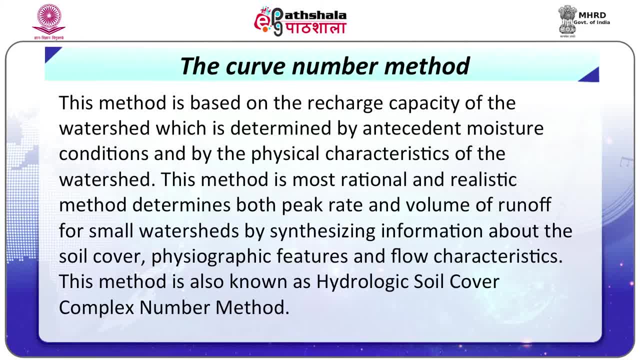 And that test is undertaken depending on or after exception of the size of the soil in the incubator, and realistic method determine both peak rate and volume of runoff for small watershed by synthesizing information about the soil cover, physiographic feature and flow characteristics. 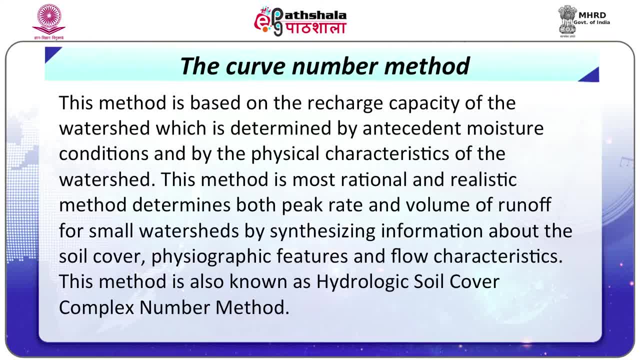 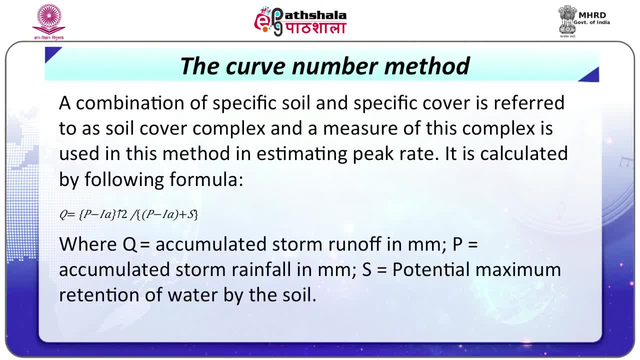 This method is also known as hydrologic soil cover complex number method. A combination of specified soil and specific cover is referred to as a soil cover complex and a measurement of this complex is used in this method in estimating peak rate. It is calculated by the following formula: where Q is accumulated, storm runoff in mm. 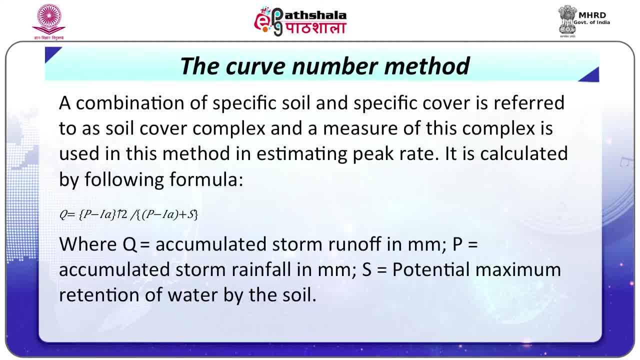 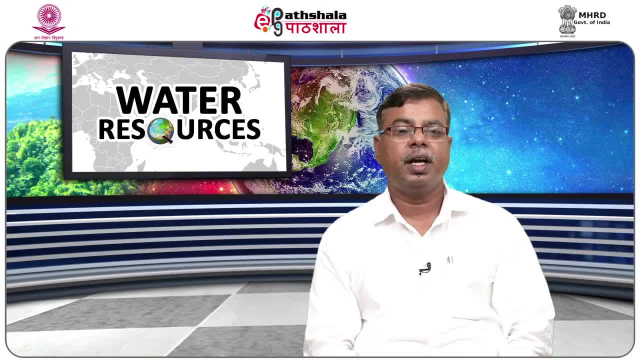 P is the accumulated storm rainfall in mm and S is the potential maximum retention of water by the soil. To simplify the above equation, Empirical relationship between the variable S and Ia was developed from the data collected from the various watersheds in USA, resulting the following equation: 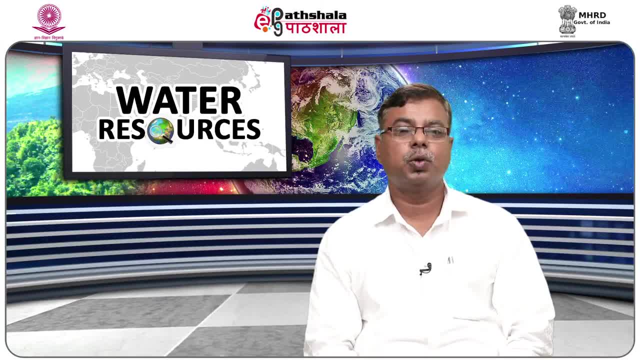 For AMC1, Ia is equal to 0.3S, AMC2, Ia is equal to 0.2S and AMC3, Ia is equal to 0.1S. For Indian condition. Central Soil and Water Conservation Research Training Institute. 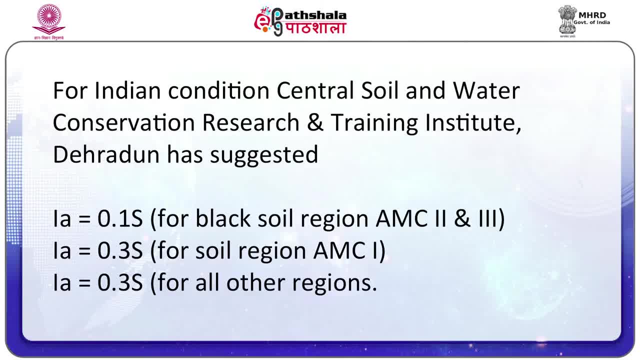 Dehradun has suggested. Ia is equal to 0.1S for the black soil region AMC2 and 3,. Ia is equal to 0.3S for soil region AMC1 and Ia is equal to 0.3S for all other region. 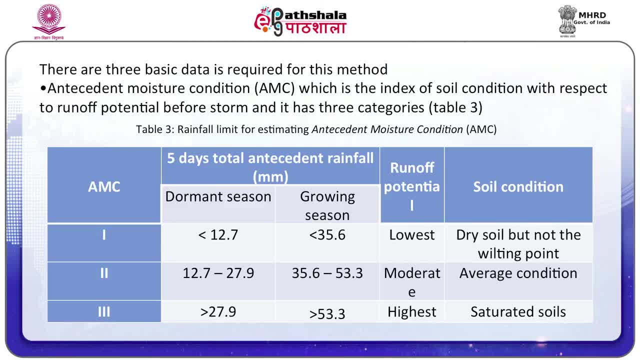 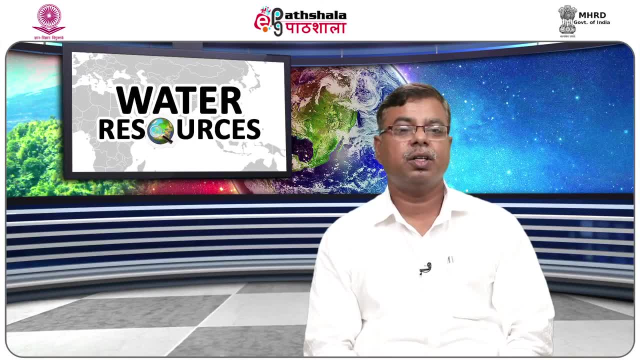 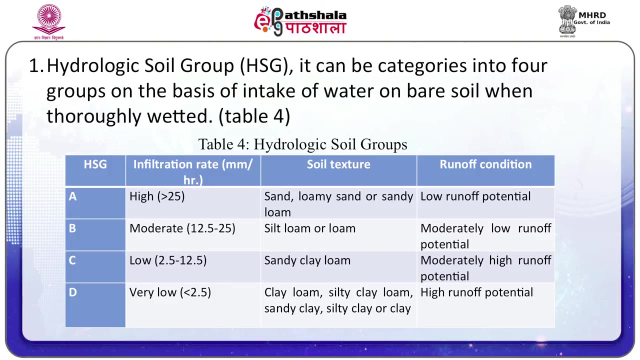 There are three basic data is required for this method. Number 1. Incident Moisture Condition, which is the index of soil condition with respect to runoff potential before storm, and it has three categories. You can see the table number 3.. The second is Hydrologic Soil Group, known as HSG. 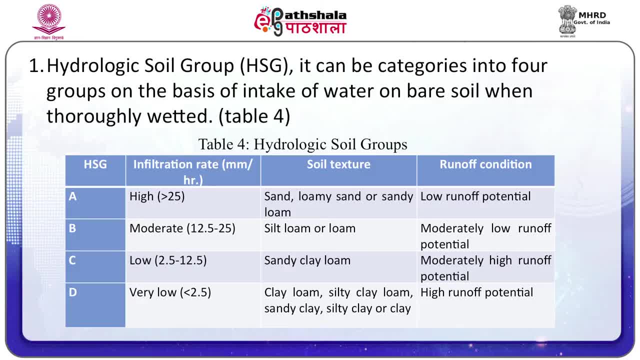 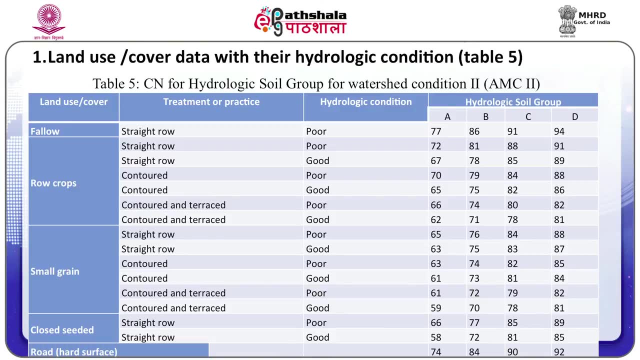 It can be categorized into the four groups on the basis of intake of water on bare soil when thoroughly wetted. Refer the table 3.. Number 4.. The land use land cover data with their hydrologic condition, as mentioned in table 5.. 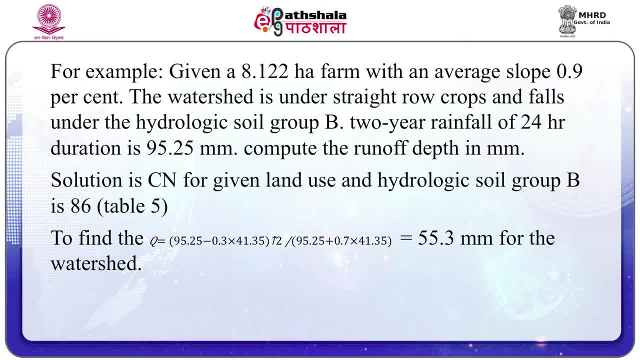 Let us see an example Given a 8.122 hectare farm with an average slope 0.9%, with watershed is under straight row crop and falls under the hydrologic soil group B, Number 3.. years rainfall of 24 hours duration is 95.25 mm. Compute the runoff depth in mm. The solution is: 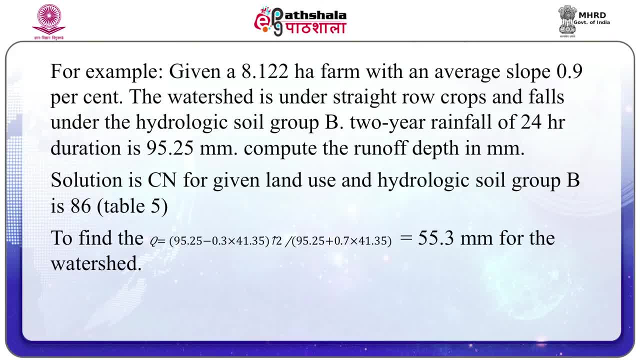 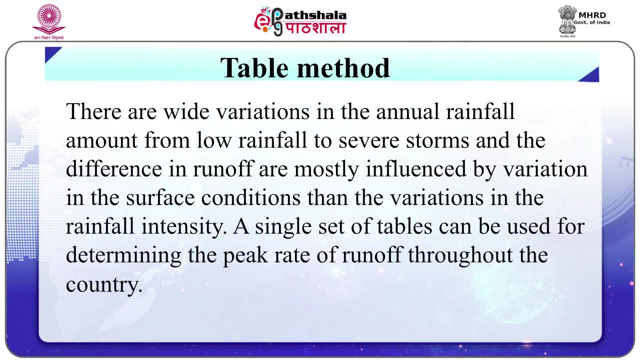 curve number for given land use and hydrologic soil group B is 86.. Refer the table number 5.. Now to find the peak runoff, that is, 55.3 mm for the watershed, by using the above formula. The next method of runoff estimation is the table method. There are wide variation in the 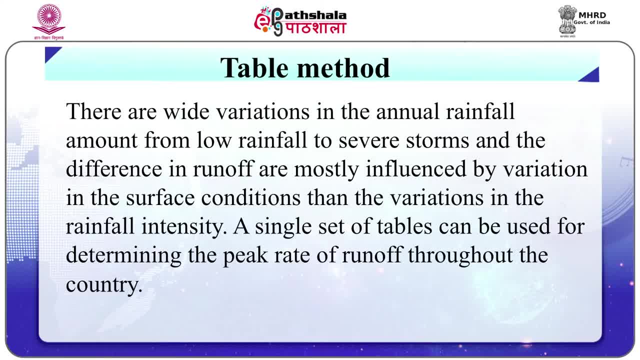 annual rainfall amount, from low rainfall to sub-strom, and the difference in runoff, and mostly influenced by variation in the surface condition, then the variation in the rainfall intensity. A single set of table can be used for determining the peak rate of runoff through the country. 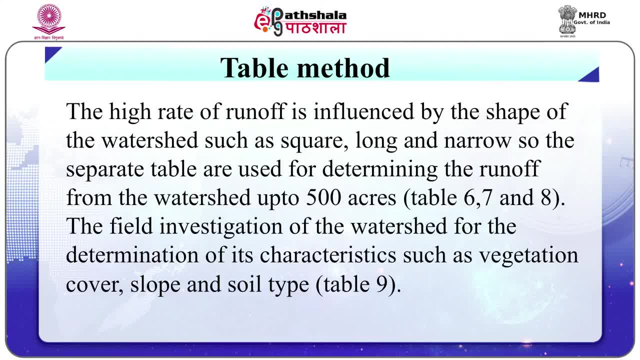 The high rate of runoff is influenced by the shape of the watershed, such as square, long and narrow, so the separate tables are used for determining the runoff from the watershed up to 500 acres: Refer the table numbers 6, 7 and 8.. 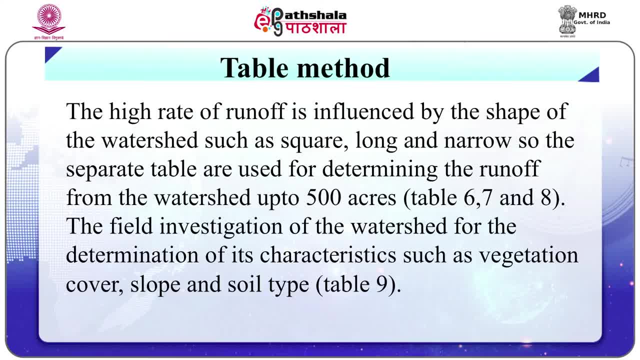 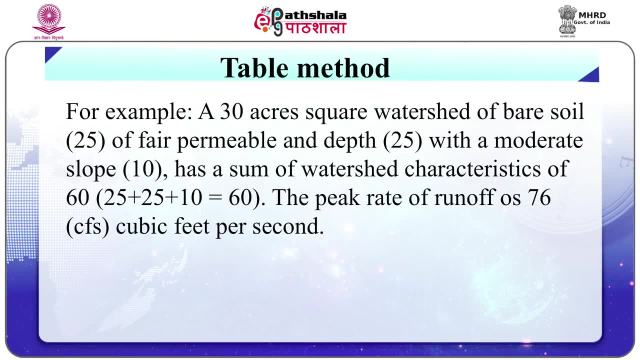 The field investigation of the watershed for the determination of its characteristics, such as vegetation, cover, slope and soil type. for that refer table number 9.. See the example: A 30 acre square watershed of bare soil of fair, permeable and depth, with a moderate slope. 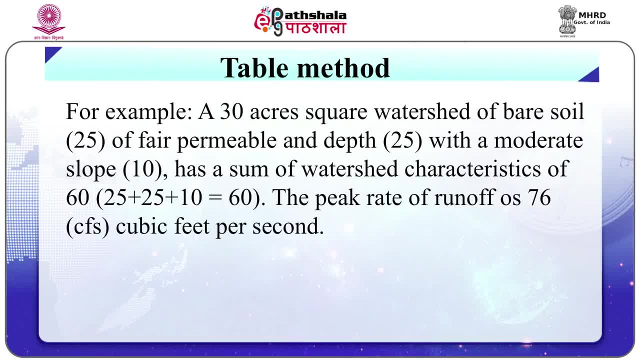 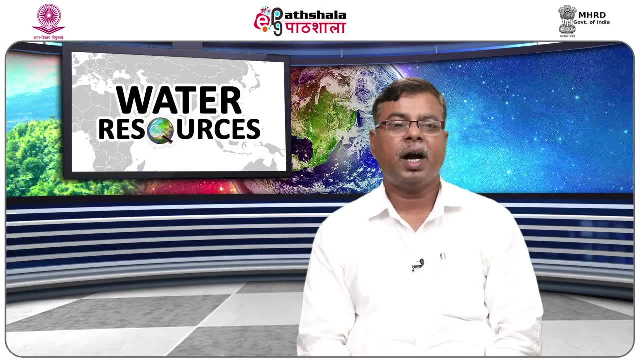 has a sum of watershed characteristics of 60, that is, 25 plus 25 plus 10 is equal to 60.. The peak rate of runoff is 76 cubic feet per second. The hydrograph: The hydrograph provides the rate of flow or peak flow at the portion in the time during and after storm or snow melt event. 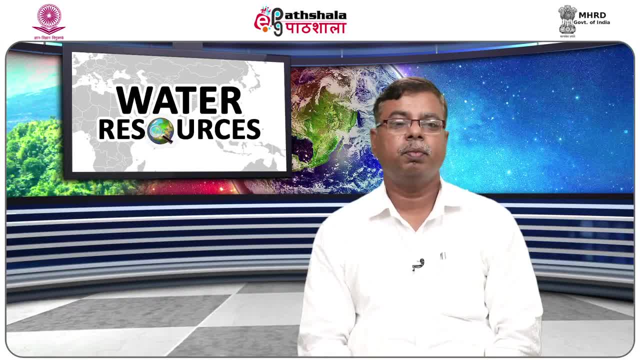 Because a hydrograph plot: volume: metric flow rate against time. Integration of the area beneath a hydrograph between two points in time, given the total volume of water passing the point of interest during the time interval. The hydrograph in figure 2 shows two graph. 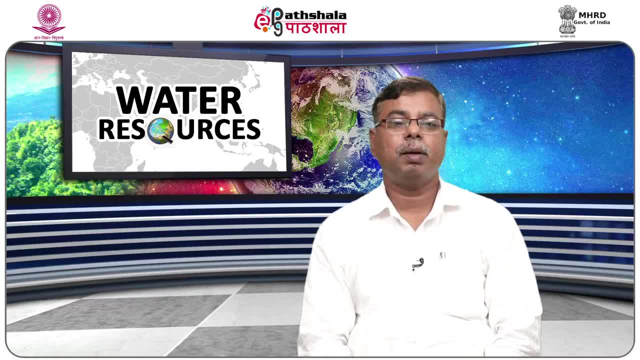 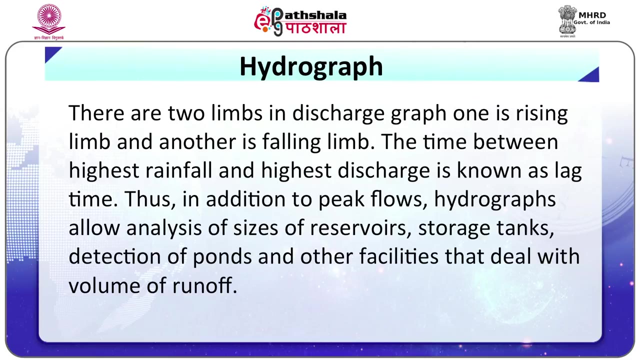 One is rainfall measurement in mm and another is water discharge in measured in cubic meter per second from watershed. The highest rainfall is a graph shown in a peak rain and highest discharge of the peak discharge. There are two limbs in discharge graph. one is the rising limb, another is the falling limb. 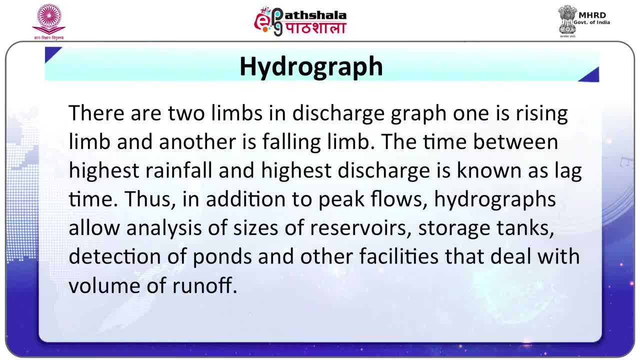 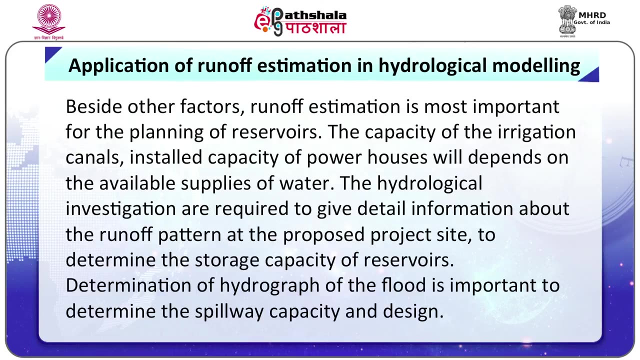 The time between the highest rainfall and the highest discharge is known as a lag. Thus, in addition to peak flow, hydrograph allow: analysis of size of reservoir storage tanks, detection of ponds and other facilities that deals with volume of runoff. The application of runoff estimation in hydrologic modeling. 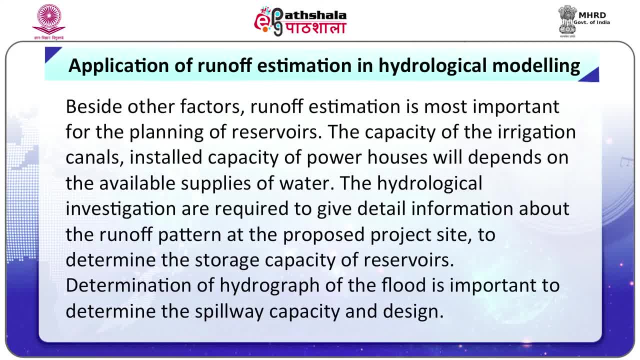 Beside other factor, runoff estimation is most important for the planning of reservoir. The capacity of the irrigation cannot be measured. Install capacity of powerhouses will depend on the available supply of water. The hydrological investigation are required to give detailed information about the runoff pattern at a proposed project site to determine the storage capacity of reservoir. 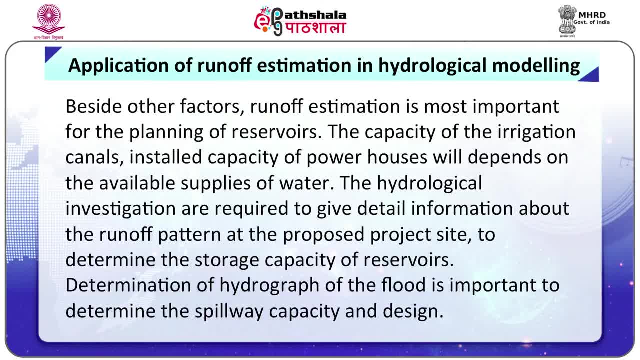 Determination of hydrograph of a flood is important to determine the space of reservoir. Determination of hydrograph of a flood is important to determine the space of reservoir. Determination of hydrograph of a flood is important to determine the space of reservoir. 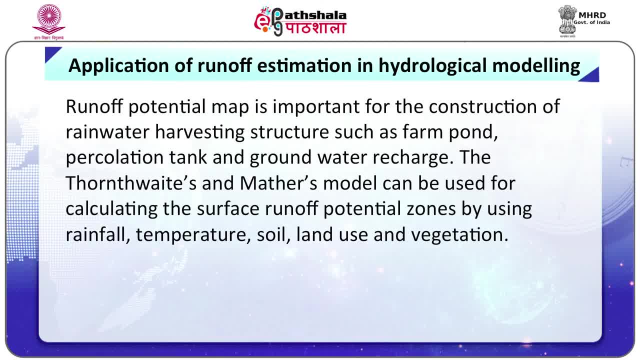 Runoff potential map is important for the construction of rainwater harvesting structure, such as farm ponds, percolation tanks and groundwater recharge, such as farm ponds, percolation tanks and groundwater recharge. The Thorbent and Mathurst models can be used for calculating the surface runoff potential zone. 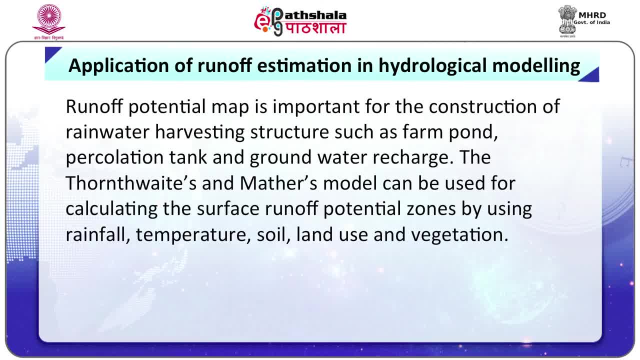 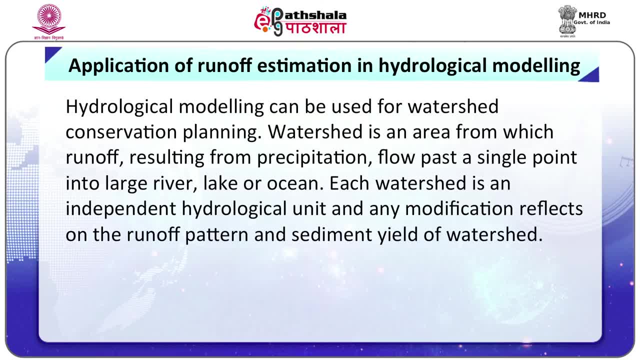 by using rainfall temperature, soil, land use and vegetation. Hydrological modeling can be used for water flowτη, For Electricity- all the smart energy of the water that we Rindt theαν For watershed conservation planning. watershed is an area from which runoff, resulting from. 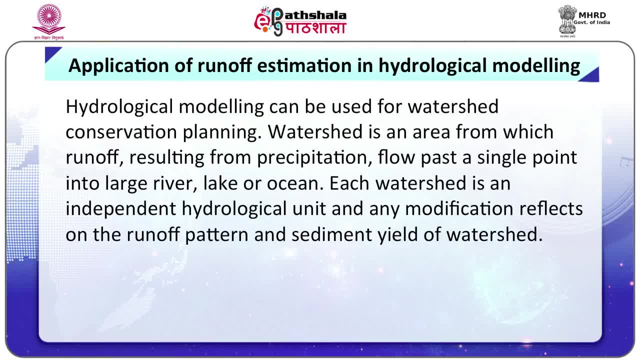 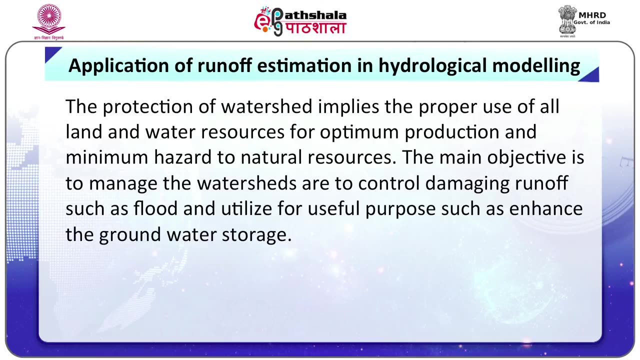 precipitation flow past a single point into large river, lake or ocean. Each watershed is an independent hydrological unit and end modification reflects on the runoff pattern and sediment yield of watershed. The protection of watershed implies the proper use of all land and water resources for optimum.